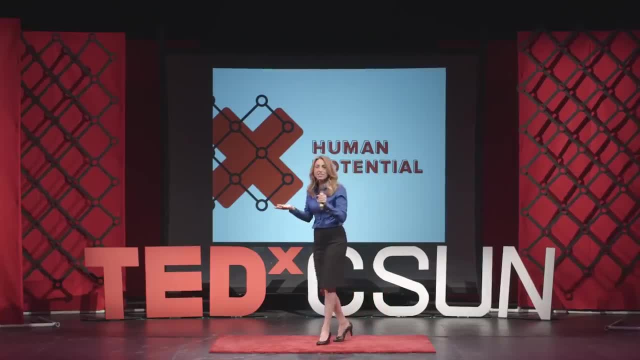 ribbons and bows. They're all different shapes and sizes. So you start to examine all of these gifts and you notice that they each have a little gift tag And on the gift tag, next to the word from, you see your own name on every single gift. These gifts are not for you, They're from you. 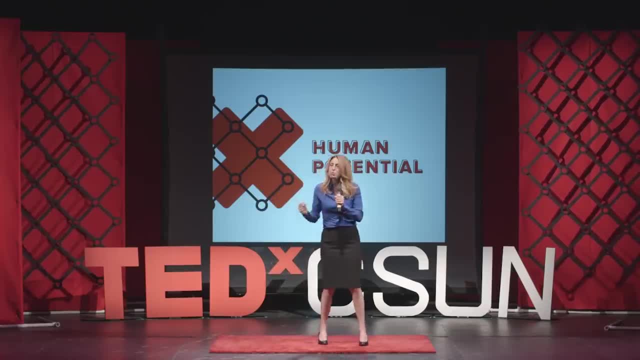 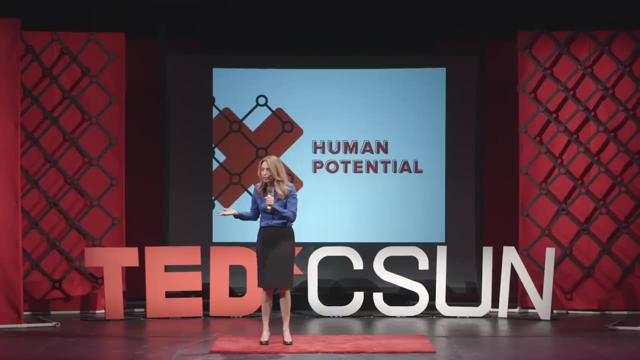 And then you look to see what names might be next to the word to, but they're all blank. None of the gift tags say who these gifts are for. So you have no idea who these gifts are meant for, And you have no idea what on earth you're going to do with them. 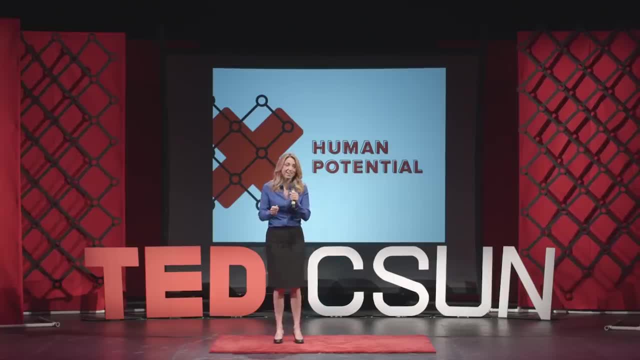 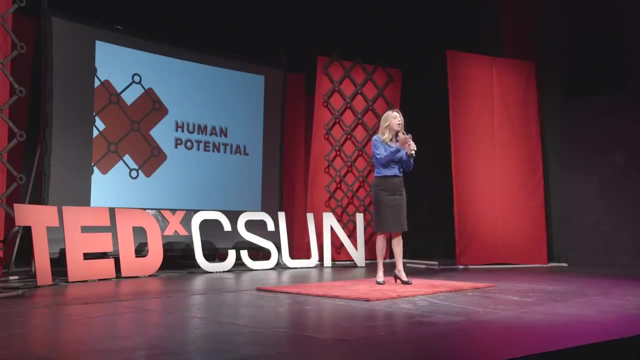 That is the question that I'm here to answer for you today. You see, these gifts represent the gifts inside of you right now, right here. They are your brilliant ideas, your unique experiences, the wisdom that only you possess. But those gifts could remain trapped inside of you forever, Undelivered and unopened. 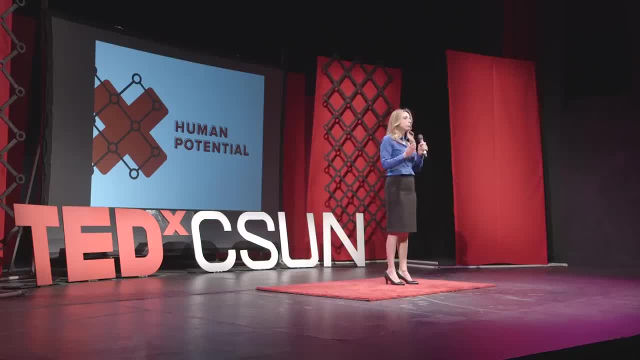 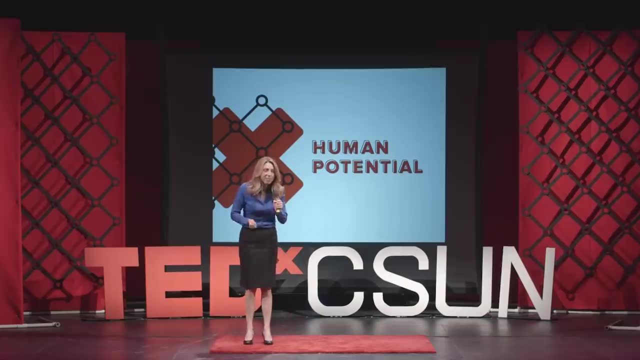 Unless you make the choice to embrace public speaking. Unless you make the choice to embrace public speaking. Yes, You heard me. If you want to reach your full potential in this lifetime, you must embrace public speaking, And it doesn't matter how you feel about public speaking right now. 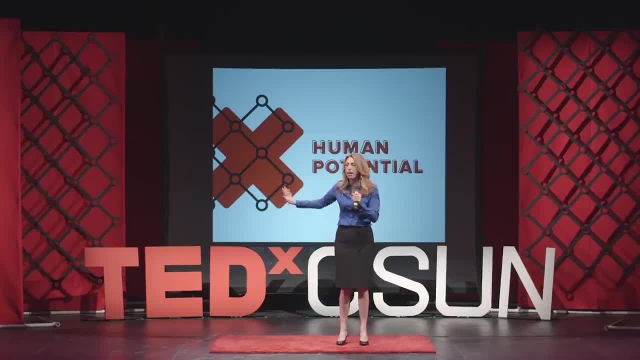 My goal is to get you to push yourself outside of your public speaking industry, because some of the gifts you bring are not yours. you're not supposed to keep them with you, But if you don't, or if you want to take them with you in this lifetime, you have no chance of remembering them. 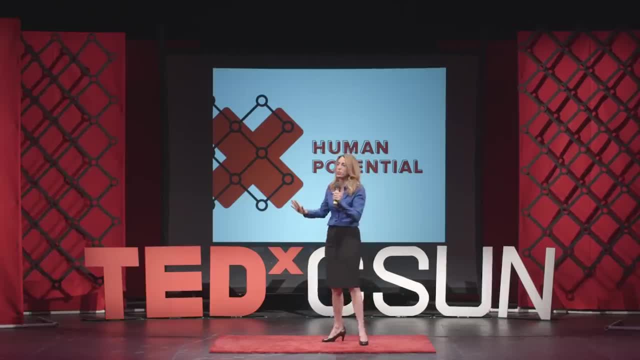 they're not wired to you, so you can't give them to people who you can't hand down their gifts. public speaking comfort zone, whatever it is for you. If you dread public speaking, I want you to summon the courage to give it a try. If you're mediocre at it, I want 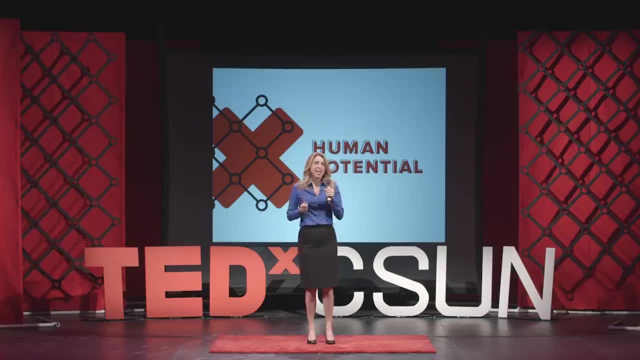 you to bring more energy and enthusiasm to it. And if you're already a great public speaker, then why don't you apply to give your own TEDx talk? It could be you here on this stage. Now, I didn't start out as a confident speaker, far. 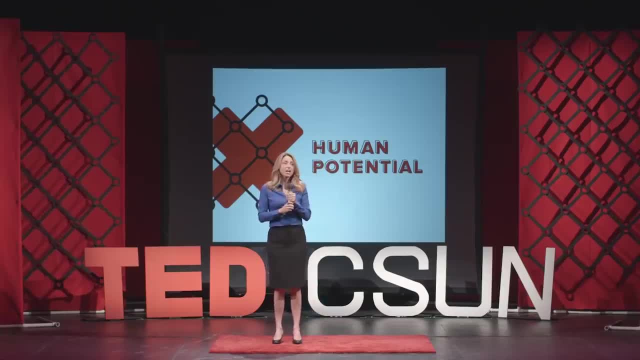 from it. I was a wreck the entire week before my very first speech in my college public speaking class. I could barely eat or sleep or think about anything else. I envisioned every possible horrific scenario that you could imagine: Projectile vomiting all over the front row. 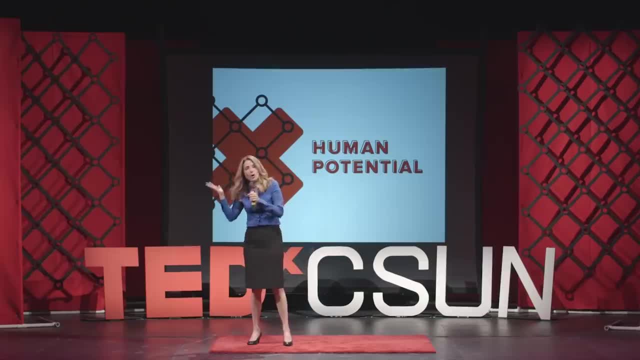 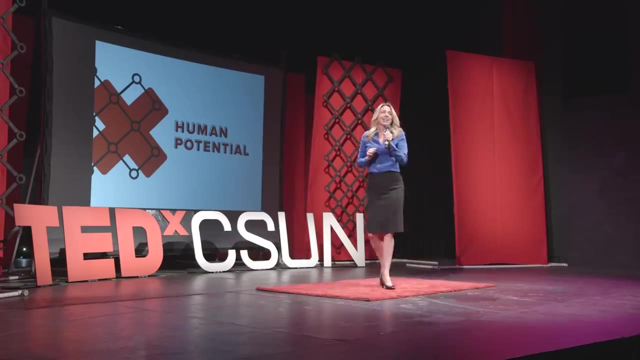 fainting and falling to the floor with a fatal blow to my head or, worst of all, standing there and forgetting everything I planned to say as the entire class howled with laughter at me. Can you relate This kind of catastrophizing by? 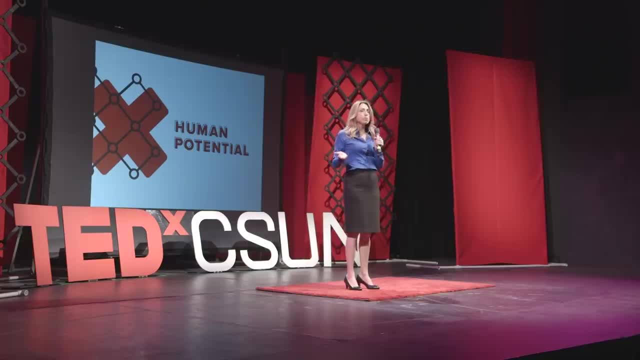 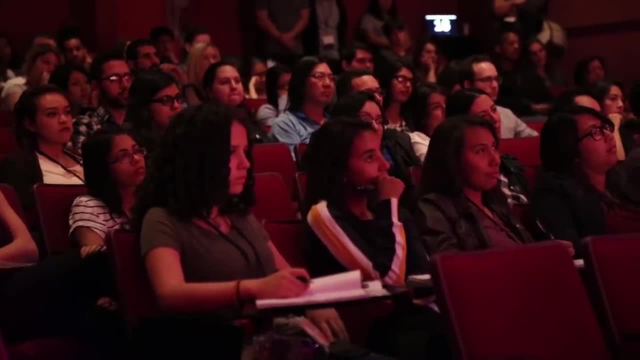 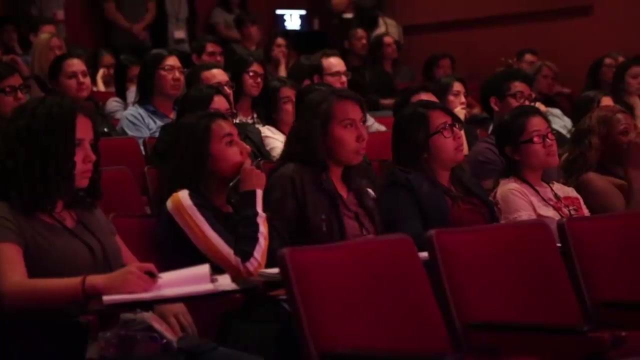 the way, is one of the reasons that psychologists label the fear of public speaking an irrational fear. The things we're so afraid of do not actually happen. So I didn't vomit, I didn't faint and I didn't forget all my points. But to be. 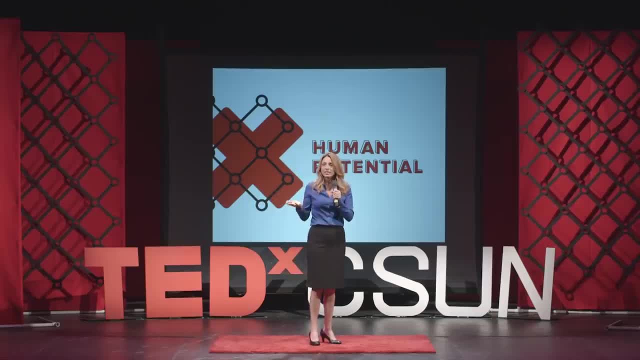 honest as self-fulfilling prophecies go, I certainly blew it. I couldn't make eye contact with a single person the entire time. I read straight from my outline with trembling hands, and I only spoke for three of the required five minutes. 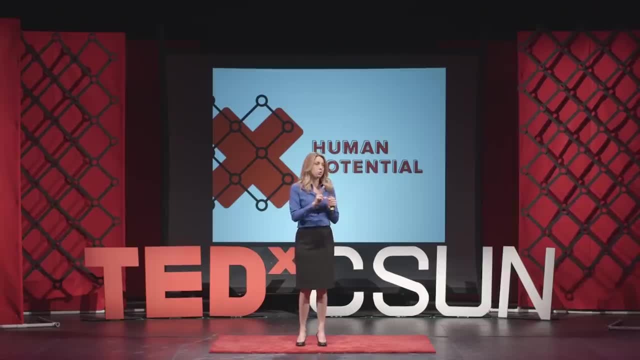 After that speech, I knew that I had two choices. I could continue to torture myself and let my anxiety run the show, or I could embark on a mission to conquer my fear and become a confident public speaker. I chose to accept that mission and it profoundly changed the course of my life. if you had told me back then that just two and a 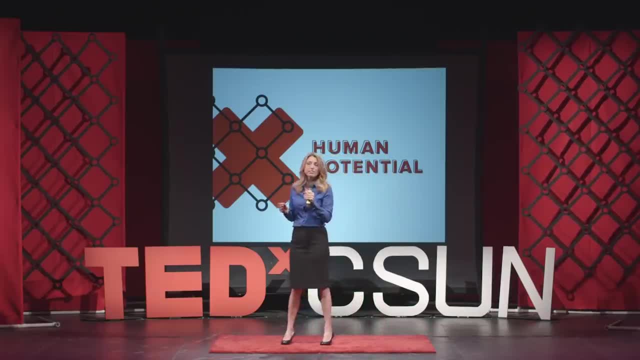 half years after taking that class I would be teaching it. I would never believed you, but it's true, or that I would happily continue to do so for 25 years and counting, and I certainly could not have imagined that that choice all those years ago would lead me to a career I love as a consultant, getting to. 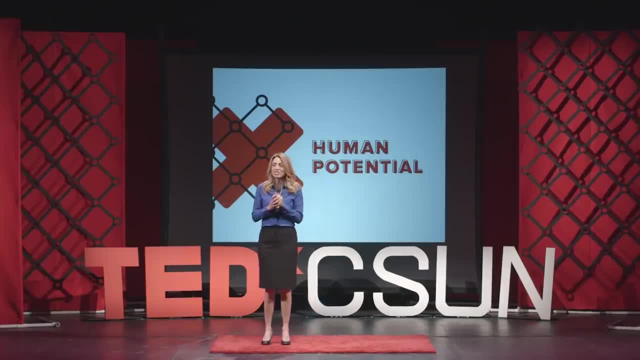 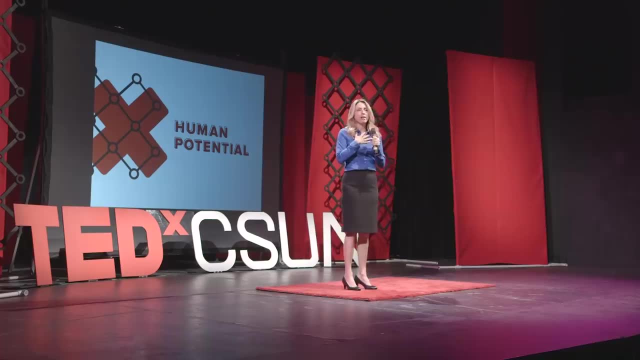 travel the world teaching people to improve their communication skills. my mission back then was to embrace public speaking in my own life so that I could unlock my true human potential. my mission now is to encourage all of you to do the same. so now that you know a little bit about my journey and my goal, 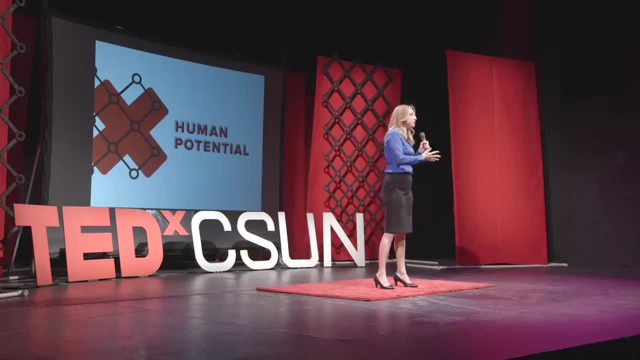 let's focus on two areas: why it's so important for you to embrace public speaking and how you can begin to do it. to answer the question why, let's look at some examples. the list of people who overcame a debilitating fear of public speaking to go on and become great leaders and entertainers is long it. 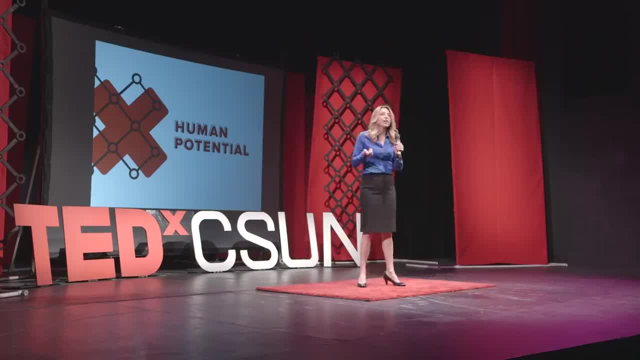 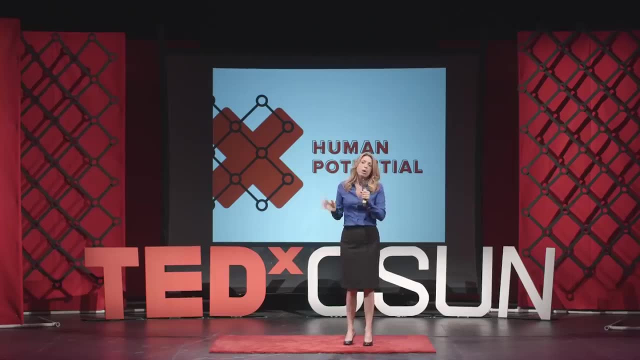 includes people such as Gandhi, Barbara Streisand, Julia Roberts, Abraham Lincoln, Warren Buffett, Tom Hanks, Nicole Kidman. I could go on and on, but you know their names right. you know all those names because those people worked hard to overcome that fear so that they could give their gifts to the world, to us. so you've heard of all. 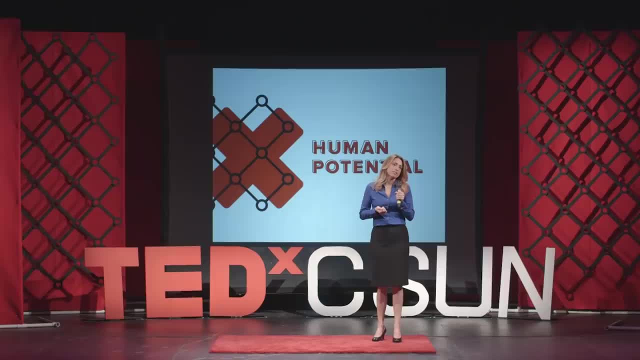 those famous people, but I bet you've never heard of Mary Ellen Peterson. she's not famous, but her story is the most inspiring one to me as a mother. especially. Mary Ellen Peterson didn't set out to be an outspoken activist, but everything changed for her in the 1970s. 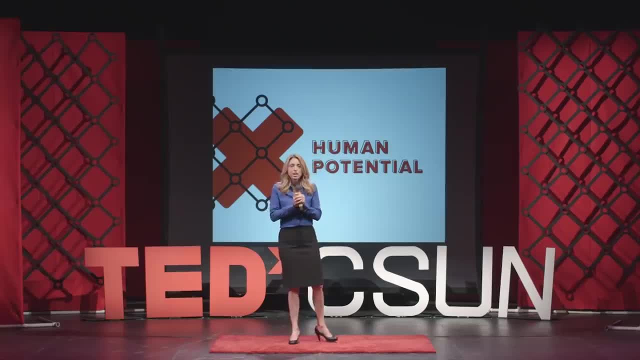 when she gave birth to a special needs baby, she joined with a small group of other mothers to advocate for their children- other mothers of special needs babies- and together they decided to form the now nationally acclaimed nonprofit organization parents helping parents, which Mary Ellen Peterson served as the CEO of for four decades, secure in the knowledge that her gift to the world. 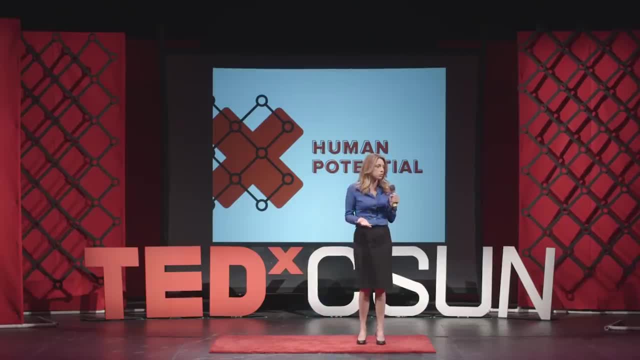 was to help families like her own with special needs children. Mary Ellen Peterson knew that she could not afford to avoid public speaking. neither can you. so you may be thinking: well, I'm not fighting to save the world like Gandhi or advocate for special needs children like Mary Ellen Peterson. 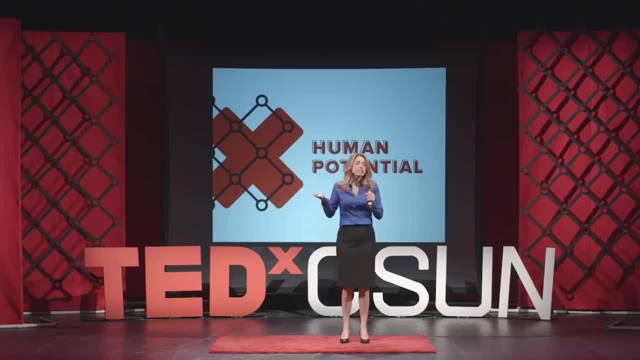 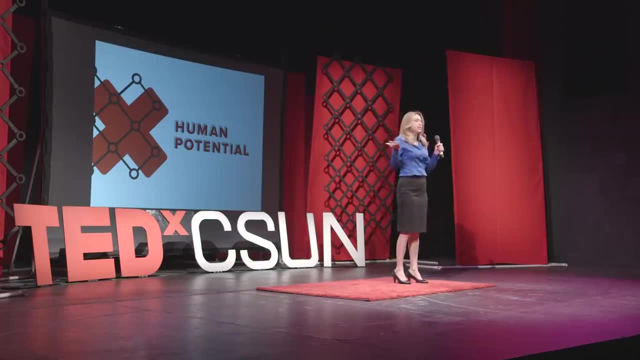 that's ok. maybe for you it's music, health, business, Finance, love, parenting, yoga, anything. No topic is too small if it's what you are passionate about, And I get it. I'm a university lecturer and trainer and coach who teaches communication skills. 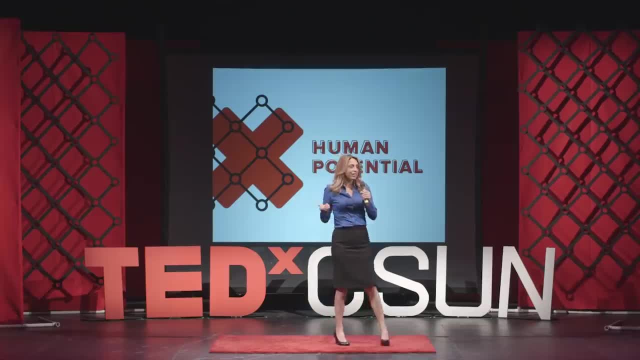 I see people's reactions. sometimes I know that a lot of people don't think that's as important as math or art or history, But I do. It's what I care most about, And so I bring all my energy and passion to every talk I give on communication skills. 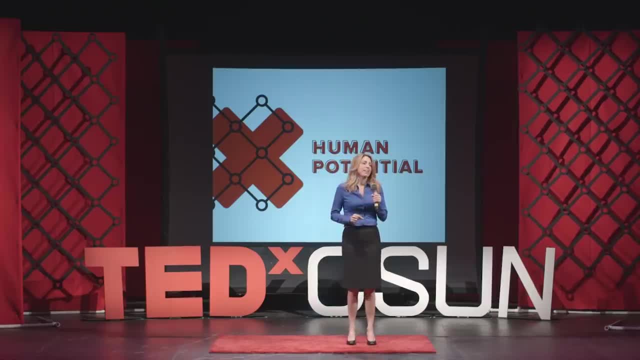 In fact, that's why I'm here today. I was asked to give three little one-hour workshops on communication skills for a student group here on campus that I had never heard of, And of course I said yes, I love to do that kind of thing. 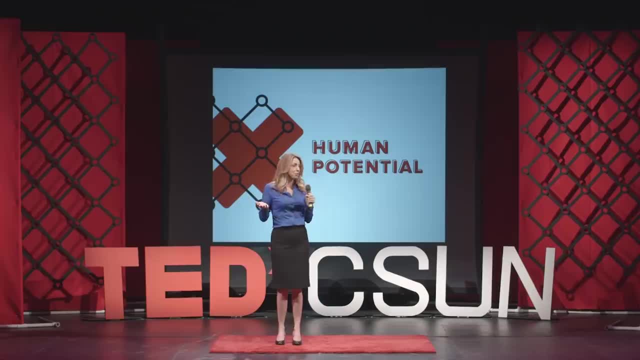 But I didn't know if any of those students would have already taken a class with me. So I spent hours coming up with all new examples and stories. I even made up a new acronym And I showed up that first day at that first workshop, so excited to be there. 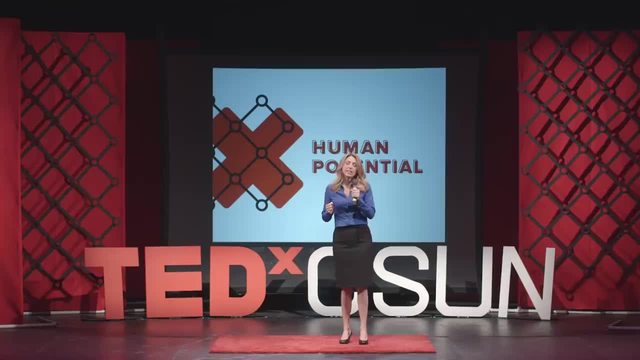 to give it my all and to engage with those students, even though I had no idea that in that audience sat the curator of this TEDx conference. It was an audition, even though I had no idea that it was, And that's why I'm here. 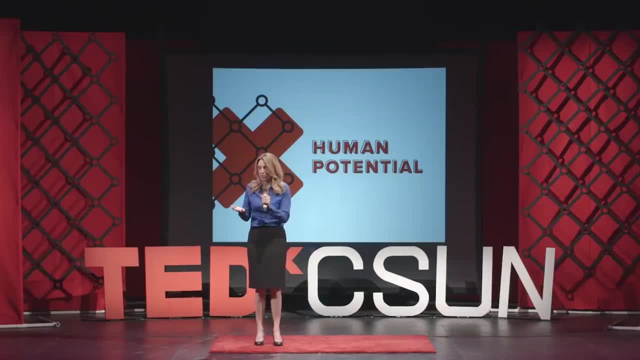 Thank you. I hope all these examples have proven to you that you- every single one of you- cannot afford to avoid or suffer through public speaking. If you do, you will absolutely miss out on opportunities to share your gifts with the world. So now let's look at how you can begin to do it. 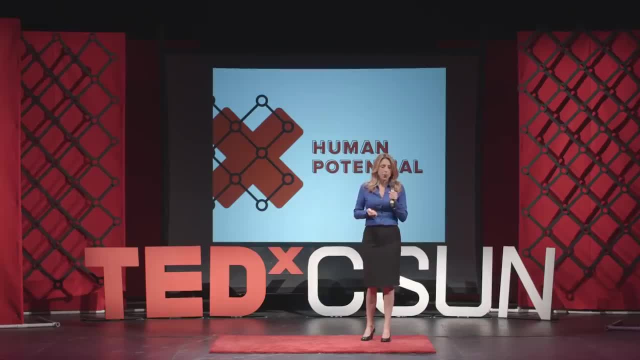 A couple of ideas regarding how you can begin to do it. It all comes down to being confident, building up your confidence. If you Google the definition of the word confidence, you'll see something along these lines: Belief in someone or something, firm trust. 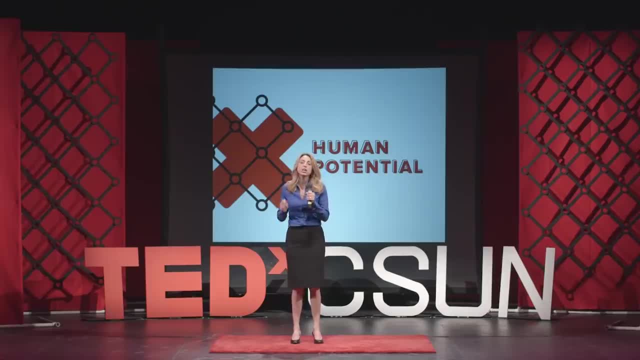 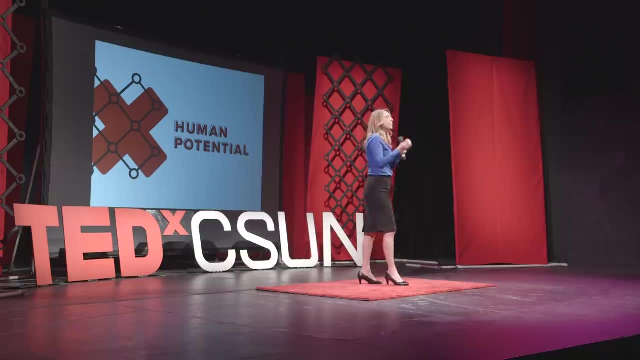 Trust is the key To become a confident speaker. you must trust yourself and your audience. To trust yourself, you've got to believe that you have something of value to share. I know you do. I just wonder if you know that you do. 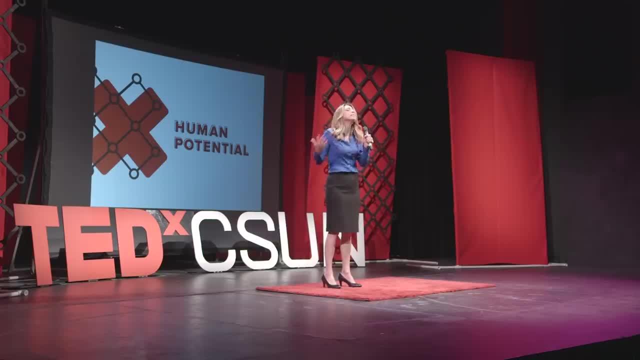 And you not only need to know that you have something of value to share, you need to believe that you already have everything you need to do it. You've done harder things in your life. I guarantee you have. One of the speech classes that I teach here on campus is for the Educational Opportunity Program. 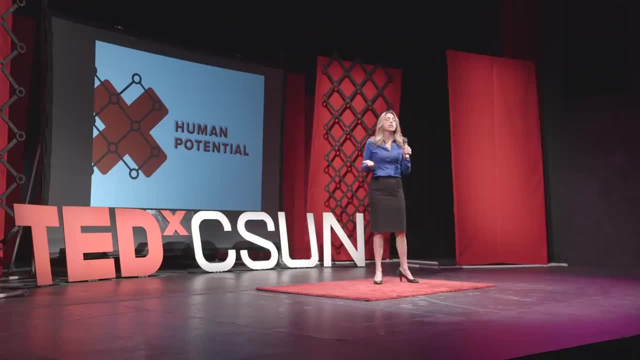 which serves historically low-income first-generation college students, And I'll never forget when I first started teaching that particular course many years ago, sitting in my office, talking to a young woman in that class, as she looked me straight in the eye and said with complete certainty: 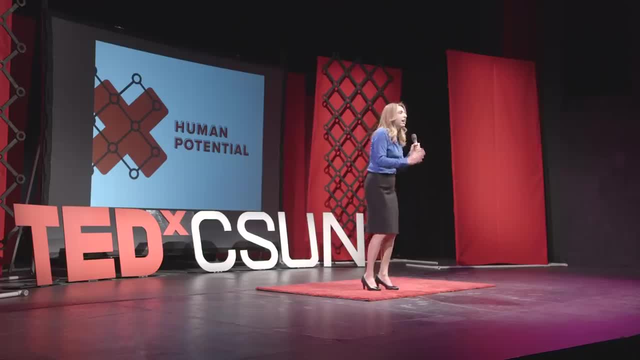 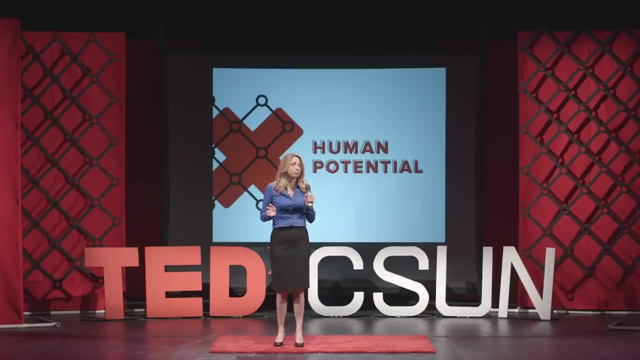 I am never going to be able to get up in front of the class and give a speech. There's just no way. She was terrified. She also shared some of her life experiences with me. She also shared some of her life experiences with me. 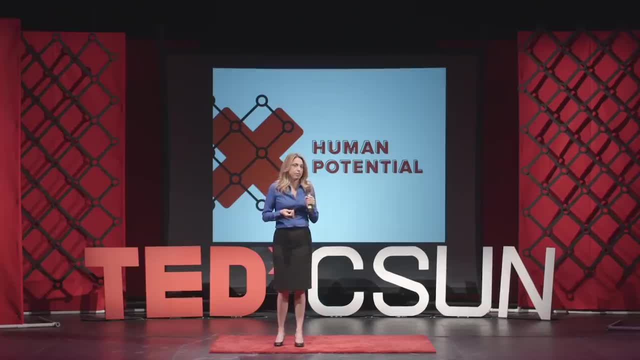 She also shared some of her life experiences with me, Things that I could not fathom: Homelessness, witnessing gang violence, domestic abuse, drug addiction, incarcerated family members. I used that information to convince her that giving a five-minute speech in front of 24 other students. 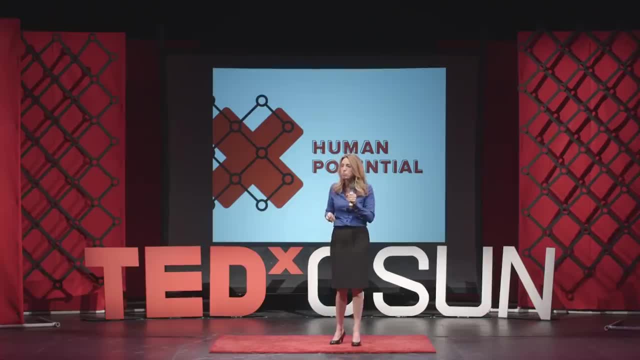 was going to be way easier than all the things she had already been through and survived in her life, That the courage it took her to break out of that kind of environment and make it to college, to a university, was way more courage than she would ever need to become a confident public speaker. 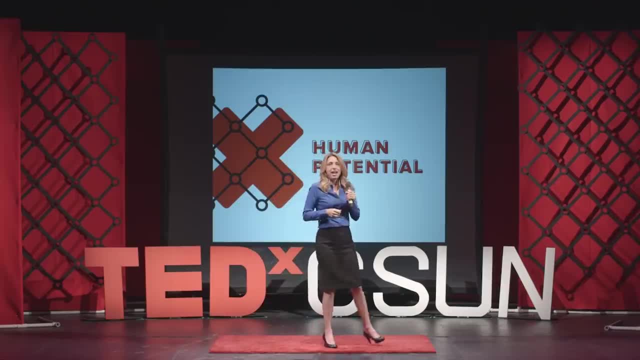 Thankfully, she believed me And it was one of the most rewarding experiences of my entire career to watch her blossom over the course of the semester into a powerful, articulate speaker And, in fact, her final speech was one of the best I've ever seen. 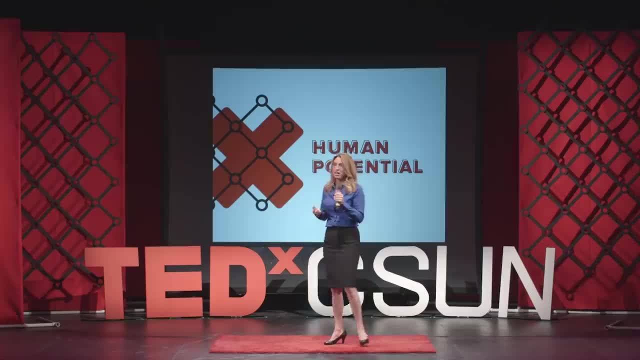 She moved us all to tears As she shared the ways that we could contribute to a world where children don't have to grow up the way that she did. I have been privileged to see hundreds of other students in the Educational Opportunity Program with similar backgrounds. 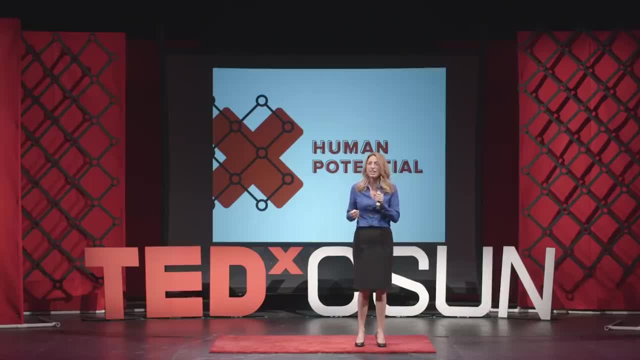 go through the same exact transformation over the years. If they can do it, so can you. Now you not only have to trust yourself. you need to trust your audience. You need to believe that the people in your audience are kind and compassionate. 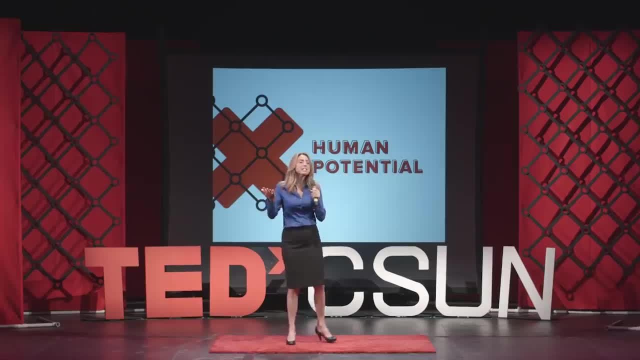 The vast majority, if not all of them, are. I guarantee you They are on your side. Aren't you on my side right now? Yes, they want you to win. Your audience is there cheering you on. Don't you do that when you're in the audience. 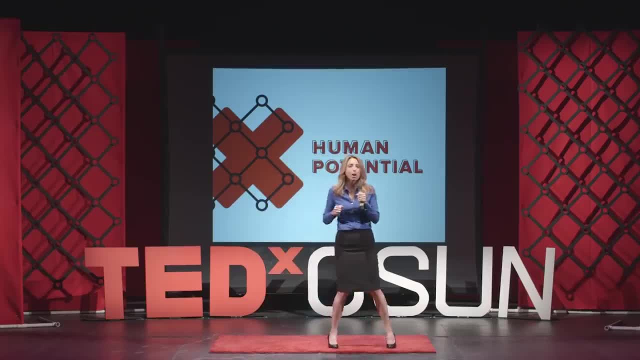 We don't sit there wishing that the speaker will be boring or will fall apart in front of us. We want the speaker to win. Remember that when you're the speaker. Not long ago, I was about to start a training program, an all-day training program for executives of a Fortune 500 company. 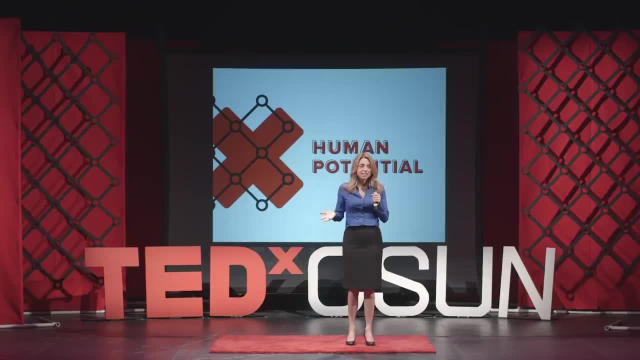 And just as I was about to begin the day, somehow my foot caught on the computer wire and I tripped right in front of them And I stumbled and I teetered and tottered back and forth and forward and back And I couldn't get my balance for what felt like forever. 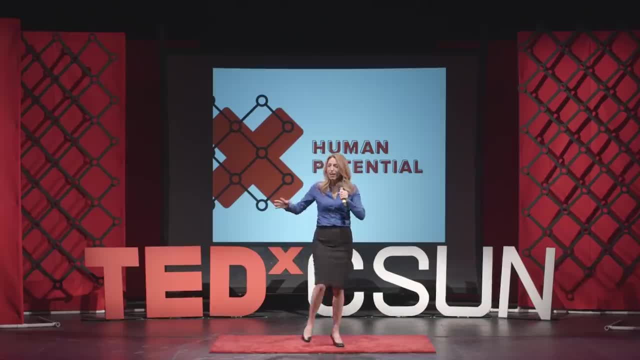 And finally, in my last attempt to steady myself, I kicked my foot out, tugged it out, tugged the wire, and watched as my laptop computer slid across the desk and slammed onto the hard floor with a bang. I hadn't yet said a word. 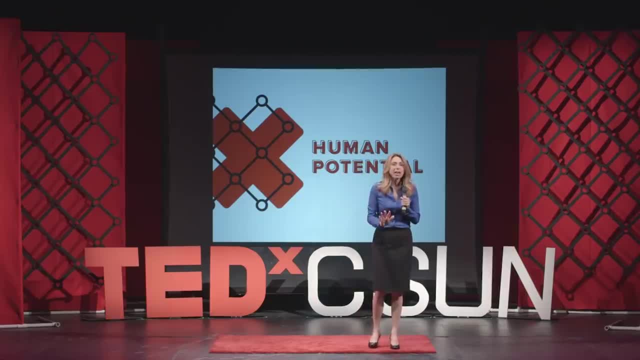 They're all staring at me. This is not the impression you want to make on Fortune 500 senior executives, right? That you're going to spend the entire day with before you've said a word. All I could do was trust that they were human beings just like me. 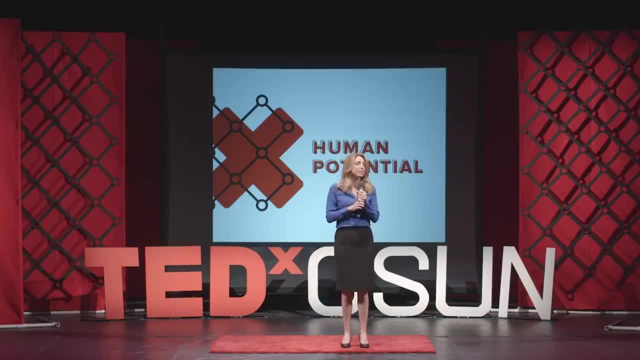 So I looked at them and all I could see on their faces was concern and empathy. That empathy feeling of, ooh, that could have been me, Or, more likely, that has been me at some point. right, We're all in this together. 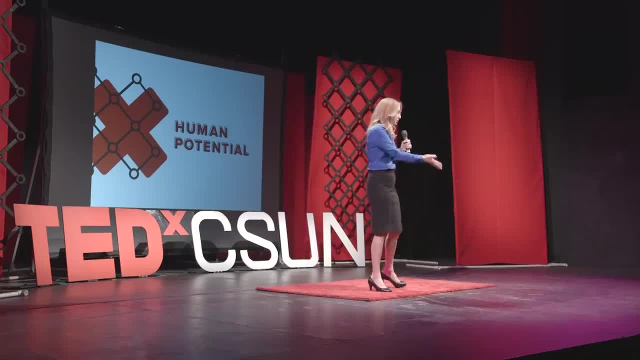 So all I could do was say the first thing that came to my mind, which was to look at my laptop and say: I hope it still works because I really like the PowerPoint slides I created for you today. And they laughed and they were happy. 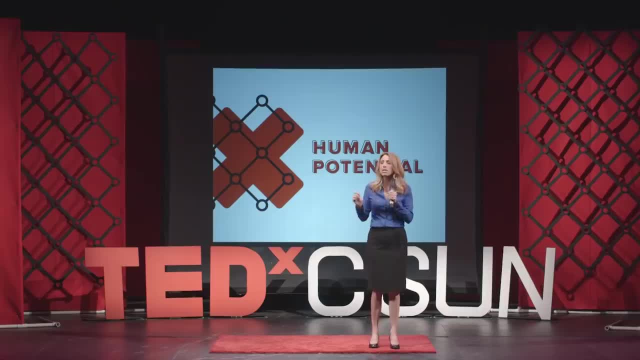 when it worked just fine. The rest of the day went great. Nobody expects perfection from you, And your audience is perfectly fine with a mistake here or there. as long as you move on, Don't make a big deal out of it. The people in your audience. 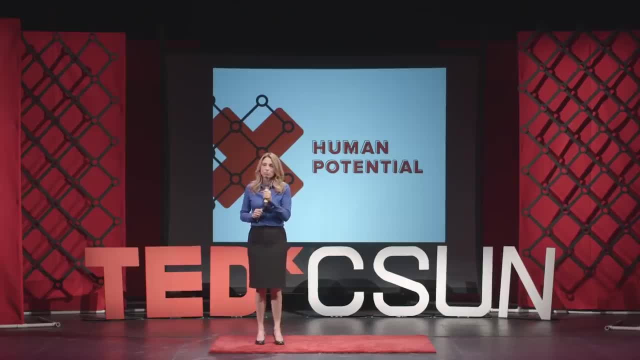 are your allies, not your enemies. Earlier in this talk, I shared with you how terrified I was of public speaking when I was in college, And I also told you about how I overcame that fear. But please do not let that lead you to believe. 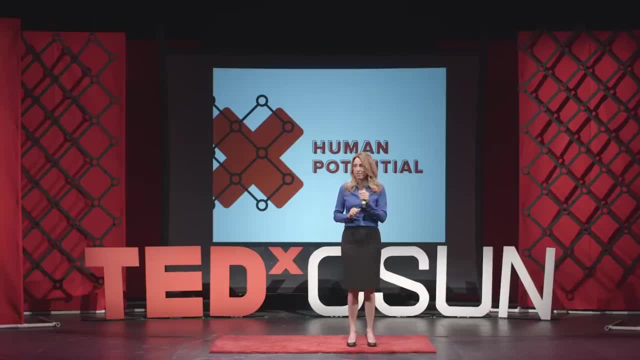 that it's always easy for me. It is not. I choose to challenge myself in new public speaking situations constantly. This, for example: I'm not used to having lights on me and cameras filming me and a microphone. This is new for me. 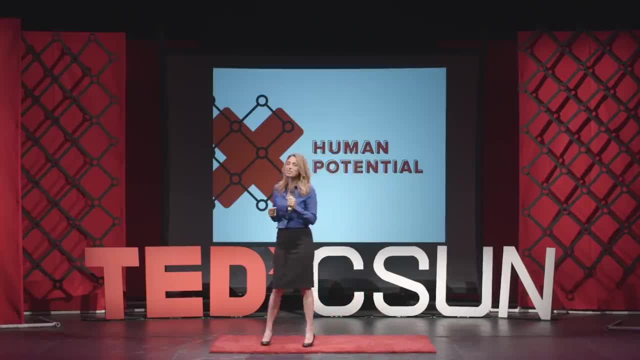 This is scary. To be completely honest with you, most of this version of this talk was composed in a complete fit of panic at 3 am a few weeks ago, And most of it was also inspired by a two-hour desperate FaceTime conversation. 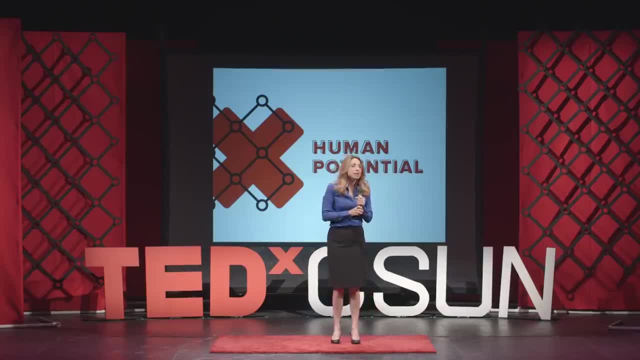 with Karina, the curator. I had spent too many sleepless nights and stressed-out days trying to figure out what to say in this talk, So I reached out to her for help And we sat there across staring at each other across our computers. 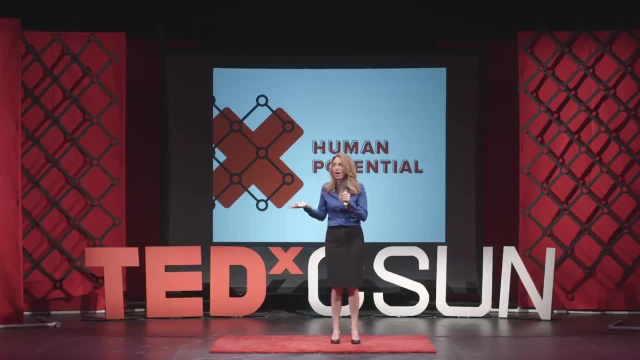 through FaceTime in our pajamas on a Saturday morning for two hours sifting through a Google Doc with my ninth crappy first draft of this talk, And I asked her to just tell me what I was trying to say And thankfully she had the answer. 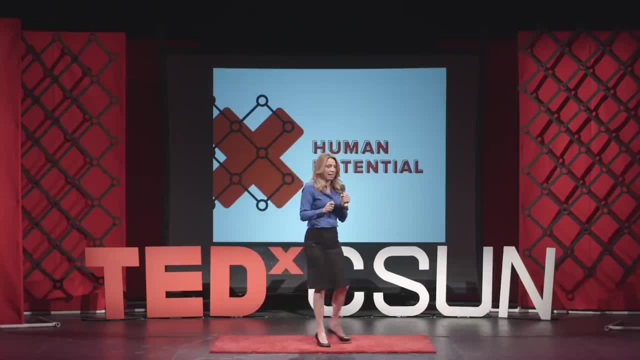 So public speaking and getting comfortable with public speaking and being a confident public speaker is required if you want to reach your full human potential. It is not optional, It's not your home that's filled with gifts, It's you, And there are people out there. 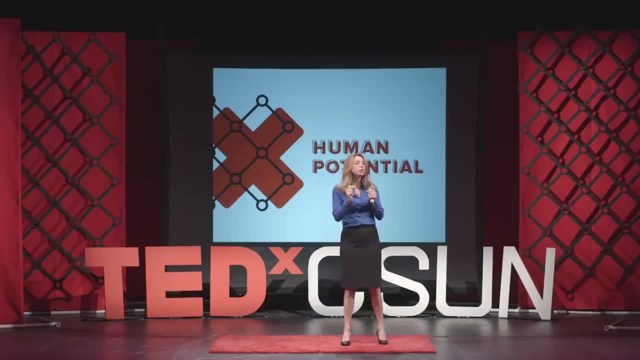 that those gifts were meant for People who need them, People who are waiting for your gifts. So the next time that you're asked to speak, the next time you get the opportunity to speak- whether it's in a meeting, at work, in a class-